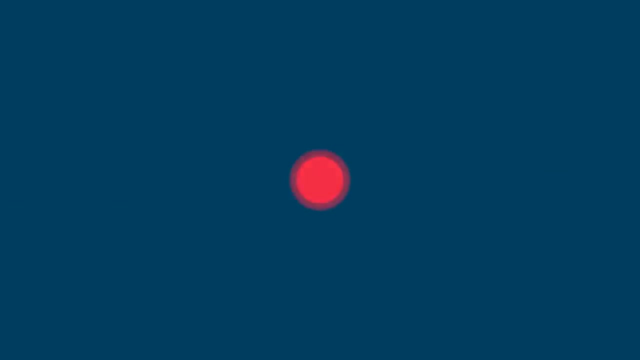 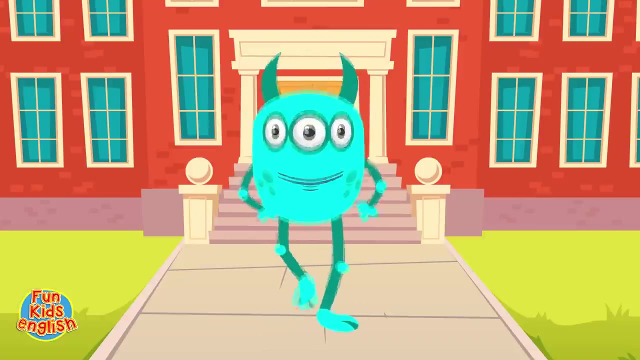 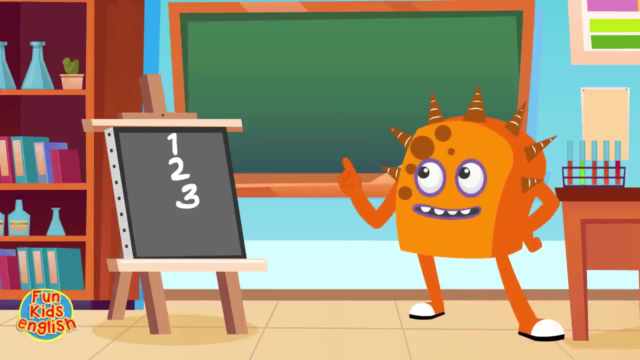 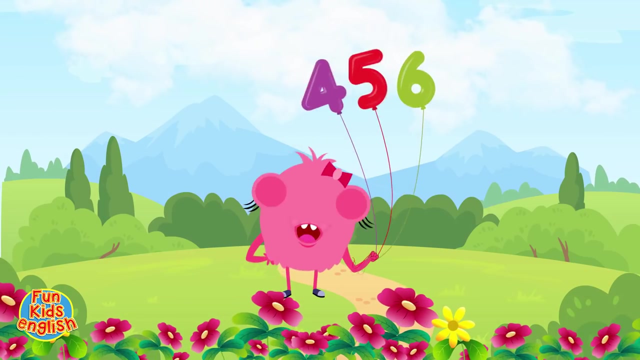 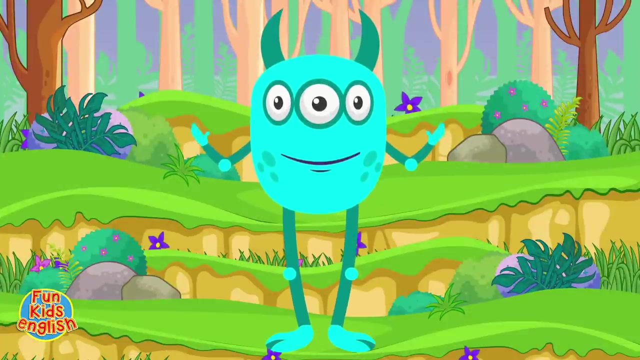 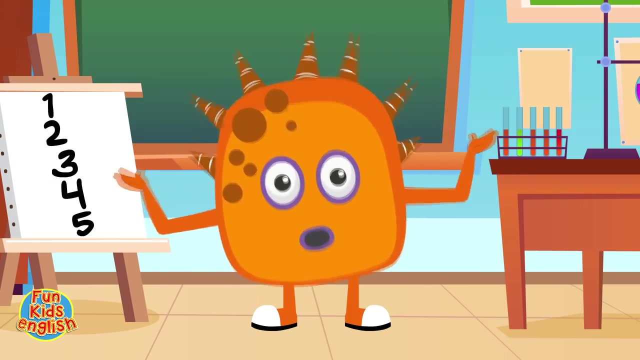 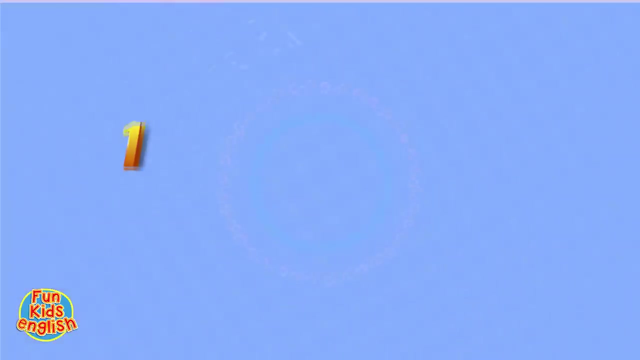 I like to count one, two, three. I like to count four, five, six. I like to count seven, eight, nine and ten. I like to count. count with my friends. Let's count One, two, three, four, five, six, seven, eight, nine, ten, eleven, twelve. 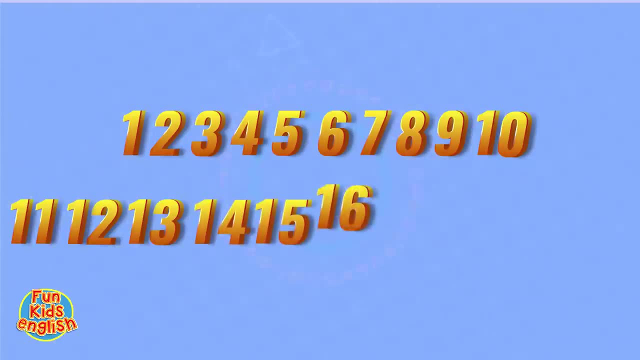 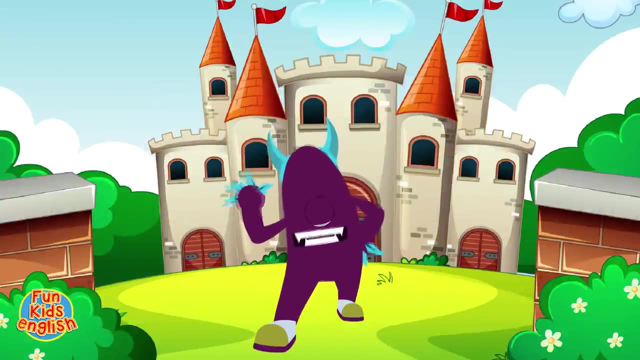 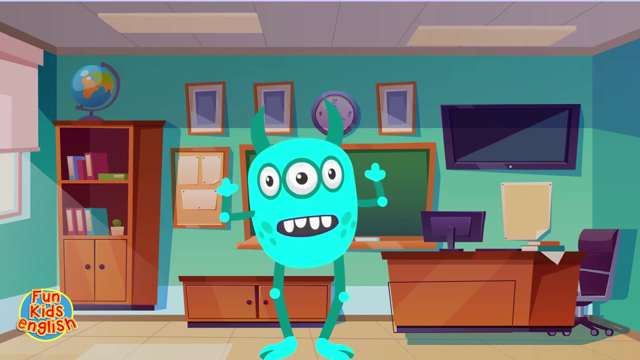 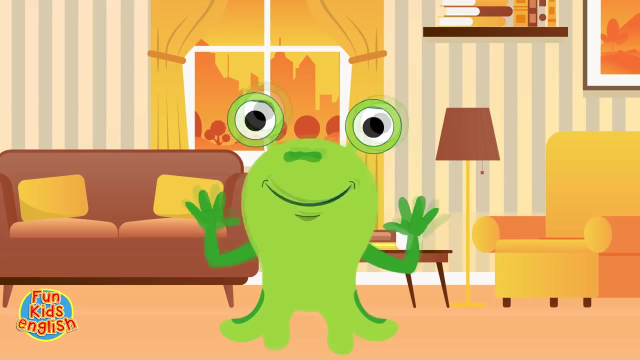 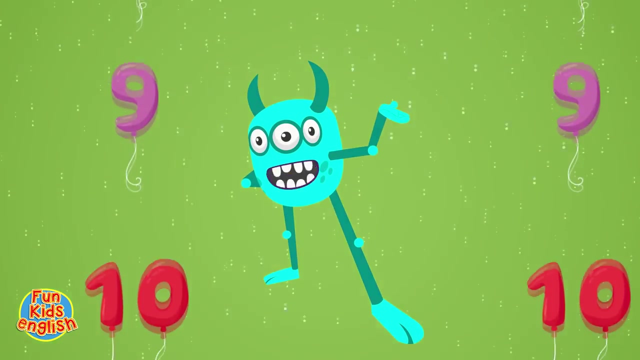 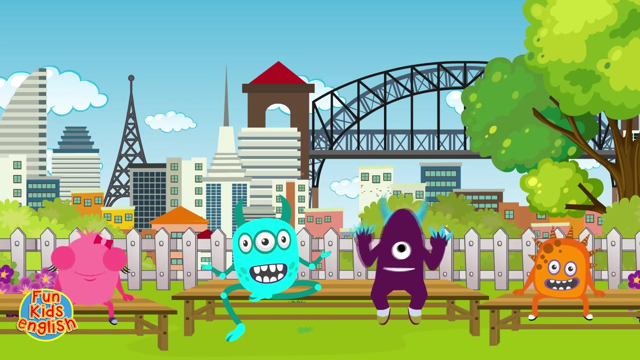 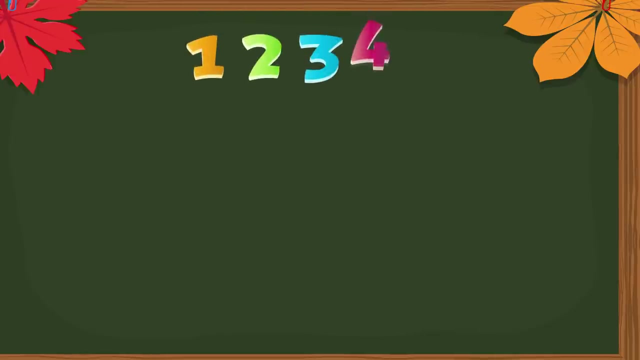 Thirteen, fourteen, fifteen, sixteen, seventeen, eighteen, nineteen, twenty. I like to count one, two, three. I like to count four, five, six. I like to count seven, eight, nine, nine and ten. I like to count. Count with my friends. Let's count One, two, three, four. 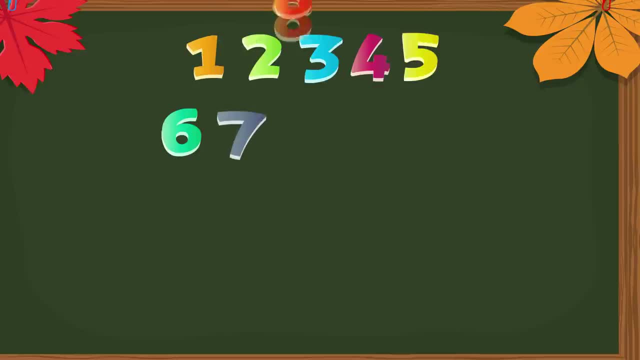 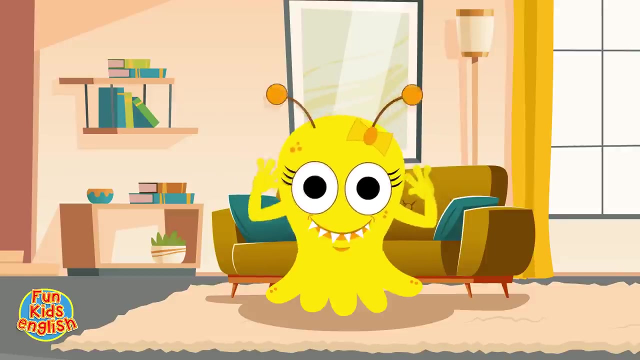 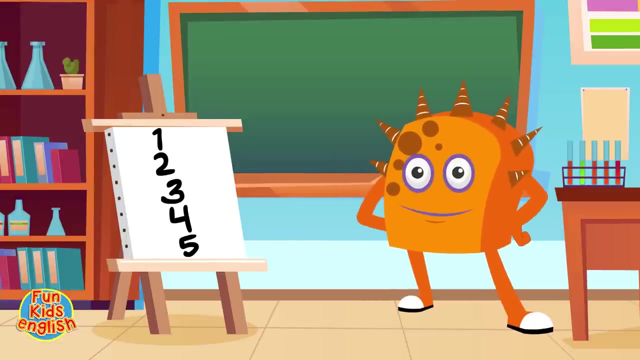 five, six, seven, eight, nine, ten, eleven, twelve, thirteen, fourteen, fifteen, sixteen, seventeen, eighteen, nineteen, twenty. I like to count One, two, three. I like to count Four, five, six, seven, eight, nine, ten, eleven, twelve, thirteen, fourteen, fifteen. 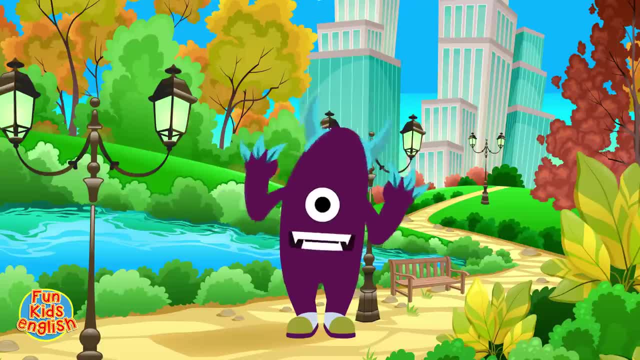 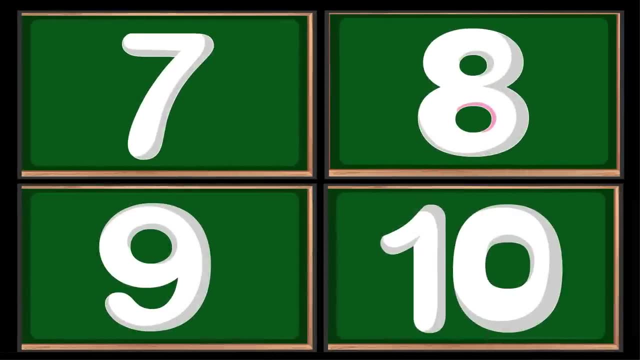 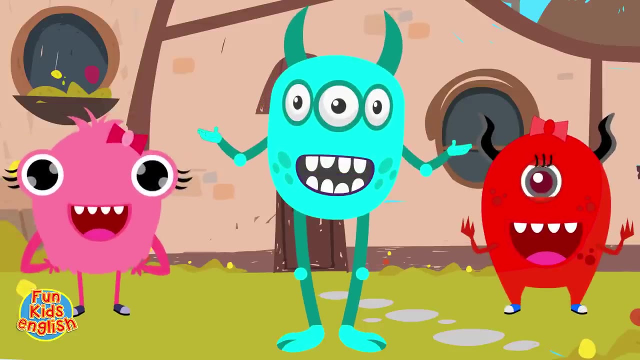 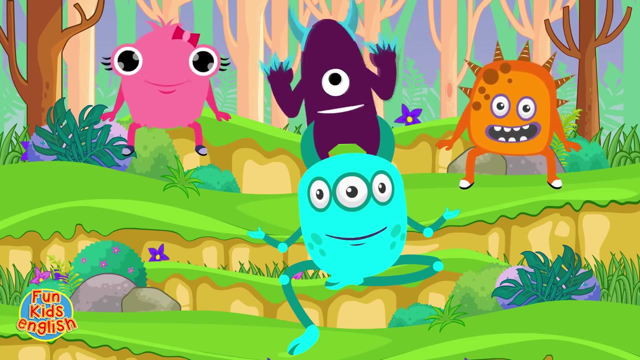 fifteen, sixteen, seventeen, eighteen, nineteen, twenty I like to count. Seven, eight, nine and ten. I like to count. Count with my friends. I like to count. Count with my friends.